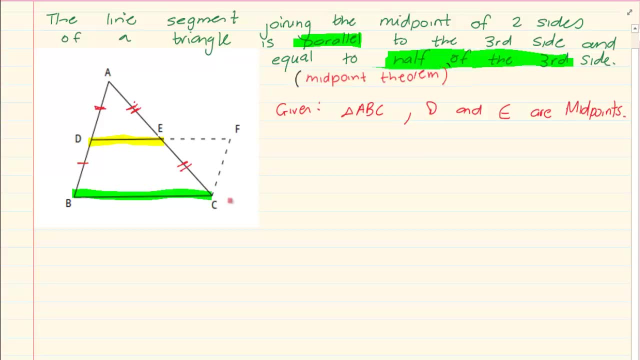 E are midpoints of AB and AC. What do they want us to prove? They want us to prove that DE is parallel to BC, And they also want us to prove that DE is equal to half of the third side. Right Now, how do we go about doing this proof? First, you need to construct, Because 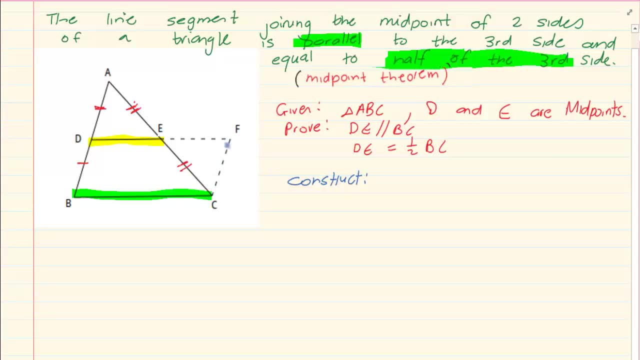 when they give you this drawing, they are not going to give you EFC. So what we are going to do is we are going to construct line FC. But look at how we are going to construct it. We are going to make it so that it is parallel to DB. So we are constructing it. 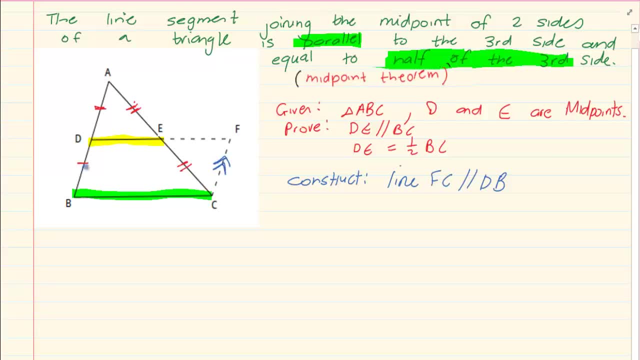 we're going to say, listen, I would like to make this line parallel to this line. Then we're going to construct line EF. Now let us start. How do we go about proving it Right? First, if you look at triangle ADE and triangle EFC, if we made it parallel, then we are saying: 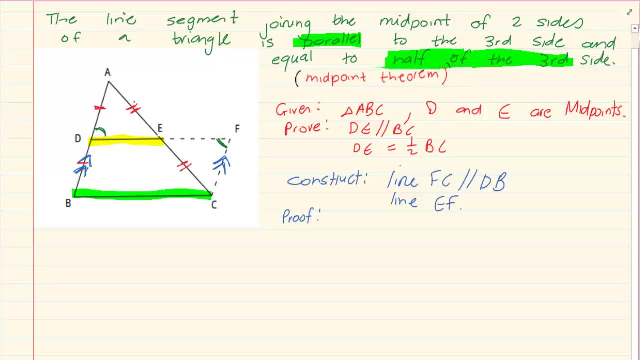 that this angle F is equal to this angle D because it's forming a Z, But there's also another Z, So from that Z I can say that the C- let's make it 1 and 2, C1 is equal. 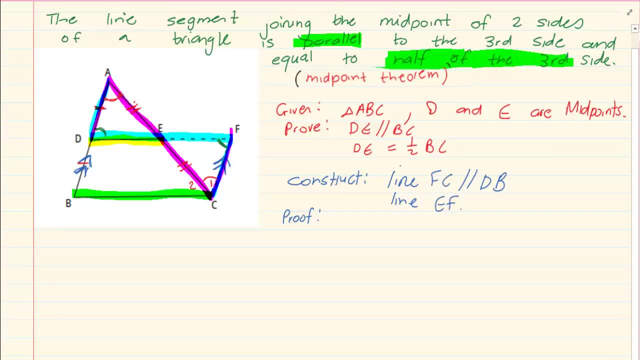 to angle A. So which two triangles are we working at? We are working in triangle, and triangle ADE and triangle CFE. What do we have? We have that angle A is equal to C1. Why It is alternate angles. And I have that AB is parallel to CF. Then I have that AE. 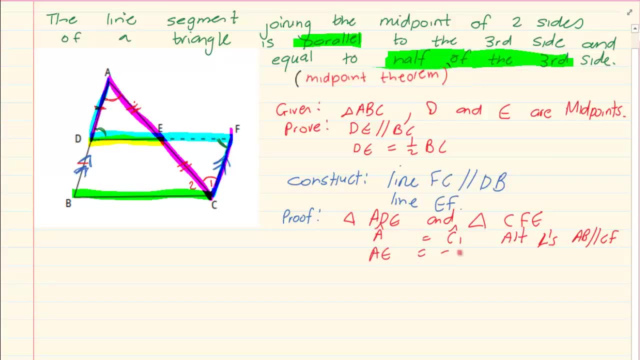 is equal to EC. That was given to us right in the beginning. They gave us that it was the mid point and since it was the mid point, it is equal. And we have the last angle, that D. let's make it D1, D1 is equal to F- Again, alternate angles. Why? Because AB is parallel to CF And I have 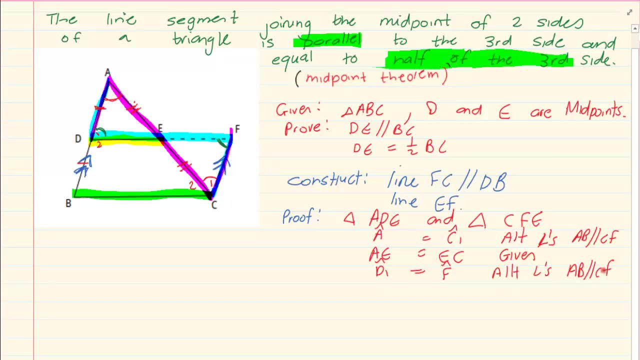 that angle A And I have that angle B And I have that angle C And I have that angle parallel to CF. now, if they parallel, then I can immediately say that these two triangles, so triangle ADE is congruent to triangle CFE, and if they are, 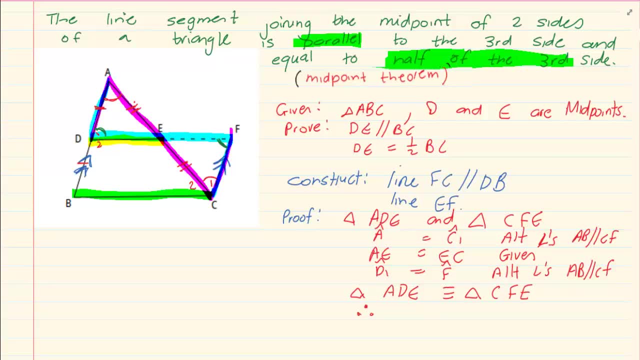 congruent, then ADE. now this is what you're saying. okay, now I prove they congruent. so if these two angles would be equal, okay, it's the remaining angle. but you should know your congruency very well. these two angles are equal, but from congruency I can say that ADE is equal to CF. ADE is equal to CF because it's a. 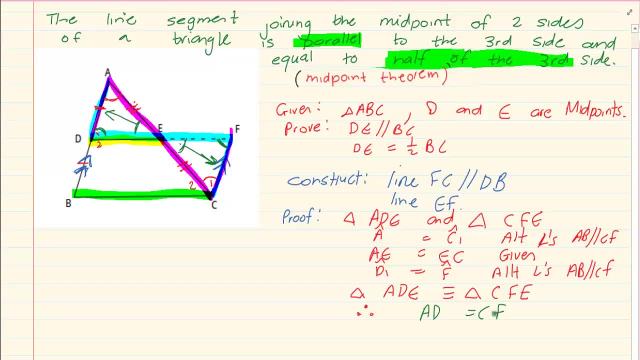 deduction from congruence. you remember what congruency? if you prove that it's congruent, then the remaining sides and the remaining angles are equal, which means ADE is equal to ADE and likewise E1 would equal to E2 and EF will equal to DE. 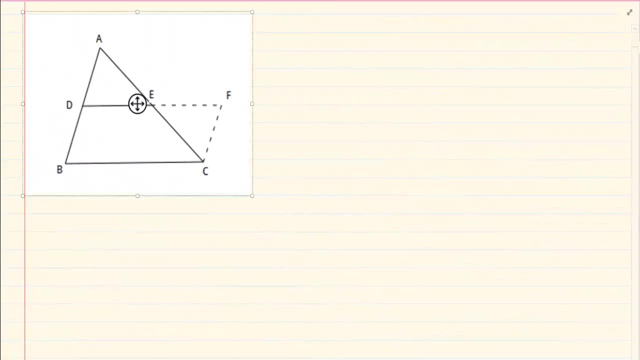 let us for what we have. we know that FC is parallel to DB. we also know that AD is equal to DB, AE is equal to EC and now, from congruency, we know that AD is equal to FC. so we know that DE is equal to EF. and remember, once you prove congruency, you